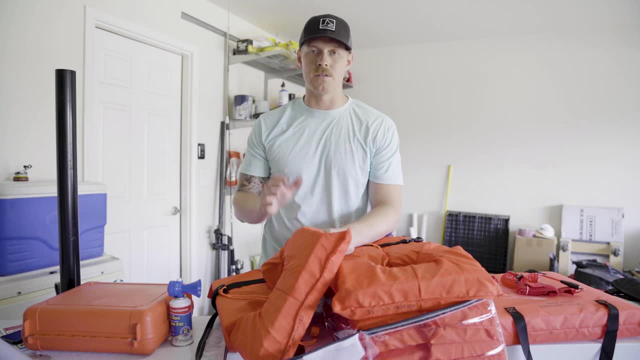 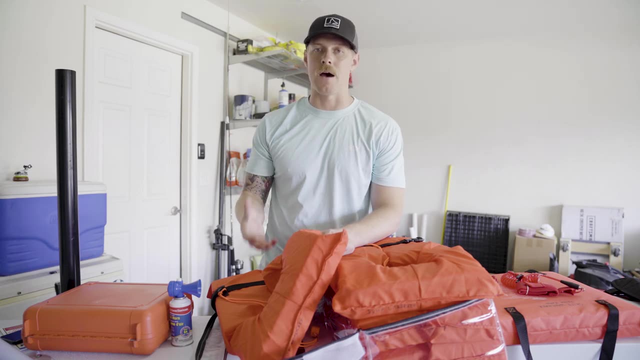 The reason being: if your boat sinks and you're floating, these will help keep your head out of the water. If someone on your boat is unconscious, it will help them keep their nose and mouth above water and breathe. I highly recommend buying some cheap little whistles and tying those on there. 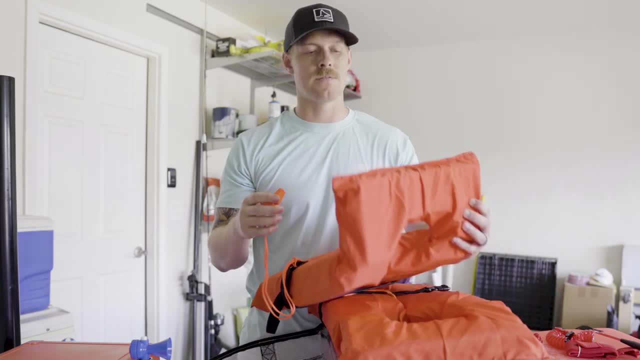 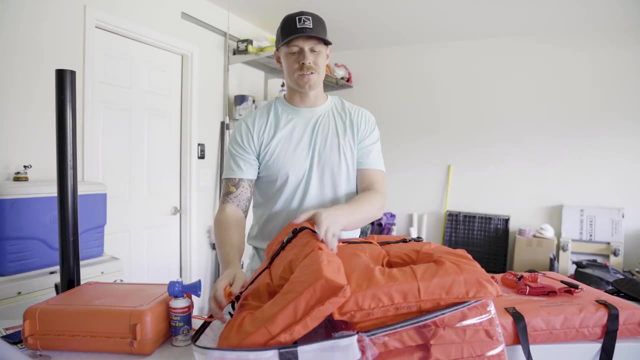 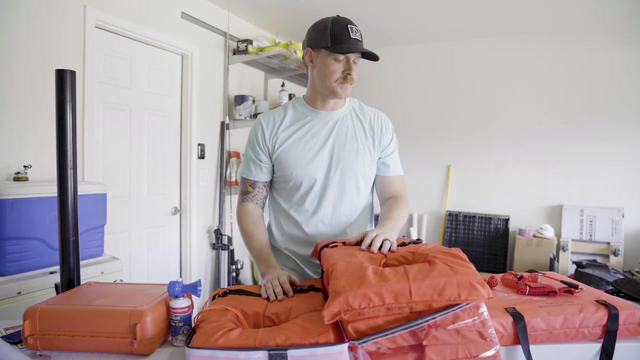 That way, everyone has their own sound signaling device. Also, go ahead and write the name of your boat as well as probably some phone numbers on there. I don't have my phone numbers on this stuff yet because, quite frankly, I don't want all you guys knowing my phone number. I'm sorry. 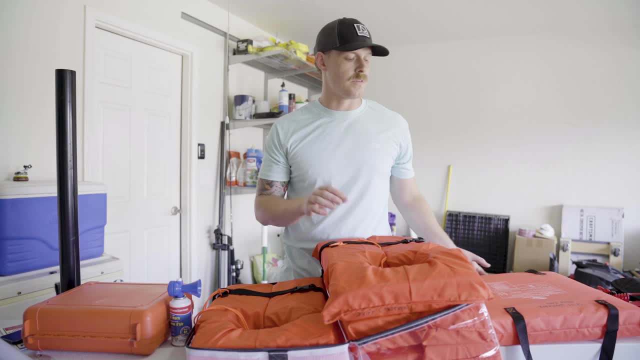 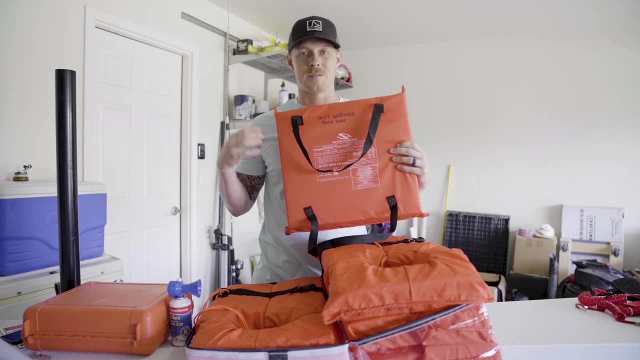 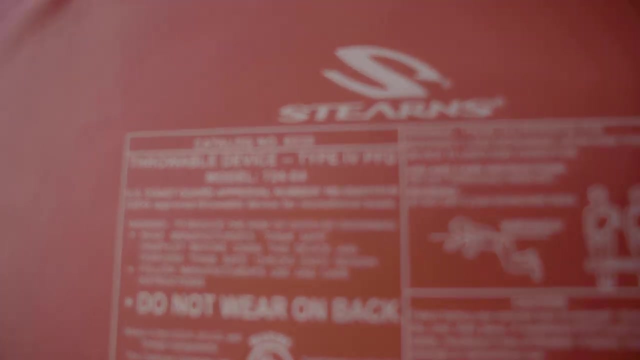 Texas requires any boat over 16 feet to have a type 4 throwable device, so here's mine. You guys probably noticed that I'm getting a lot of stuff that's orange and that's because it's highly visible. Again, name of the skiff as well as my name, and I'll probably go in and write my phone. 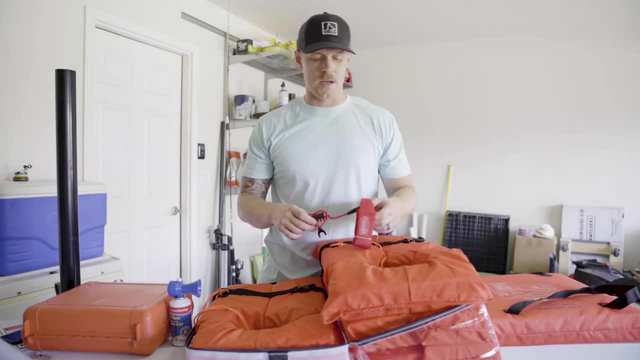 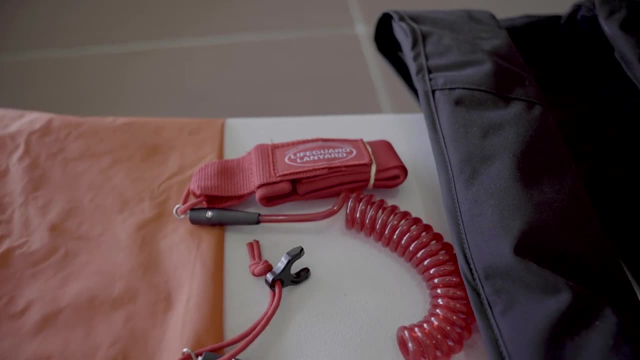 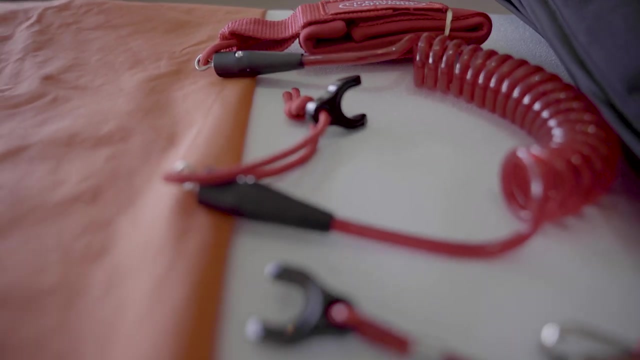 number on it in a little bit. Last thing: Lastly, the state of Texas requires you to have engine cutoff switches. Now I went ahead and got this lifeguard lanyard, which gives me a lot more room to move around my skiff while I've got the engine running. 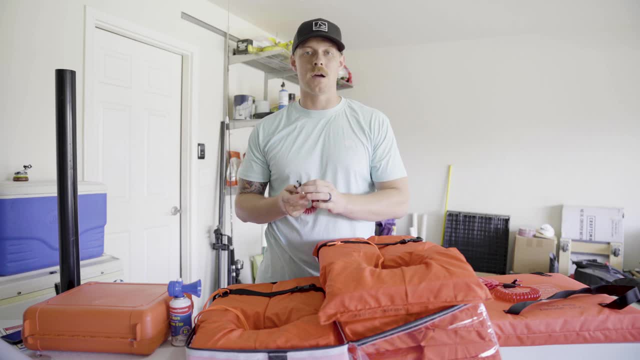 That being said, I do have a secondary cutoff switch, which I will keep on the boat. That way, if I fall off the boat while I'm operating, someone else can quickly grab this one. I'll just slide it into the motor and come and pick me up. 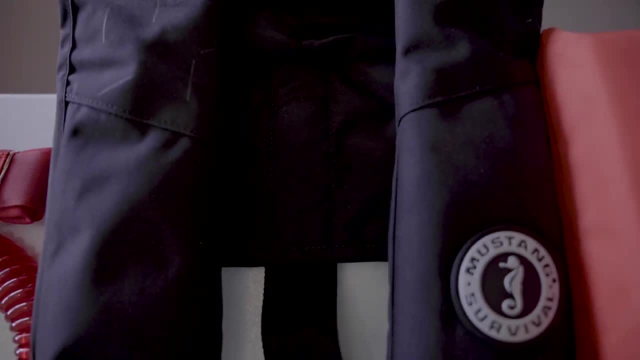 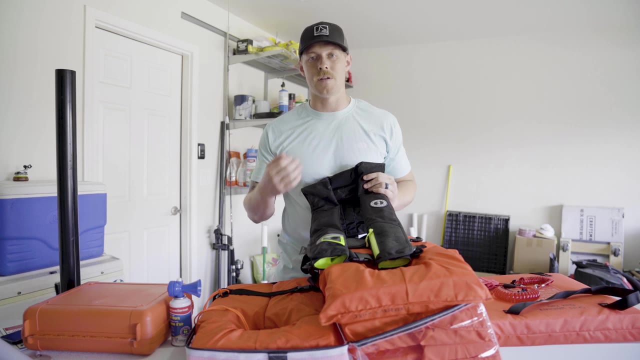 The last little thing in terms of safety equipment. I got a Mustang survival auto inflate PFD, type 2 PFD, and this is for whenever I'm operating the skiff and I'm on it by myself. That way, if something happens to me and I fall off the boat, it will automatically inflate. 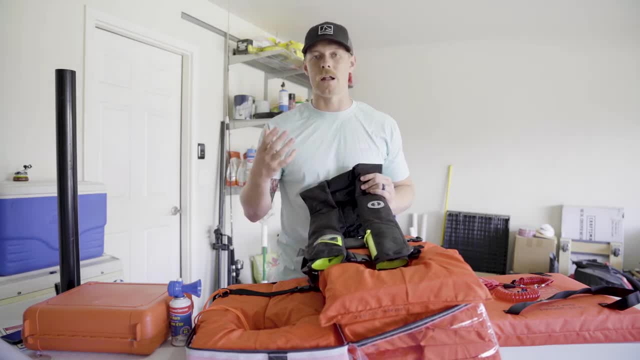 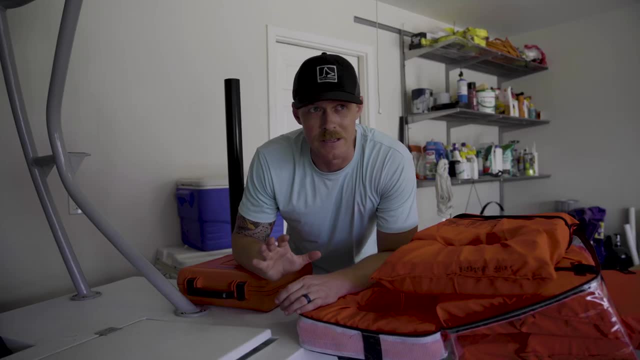 and if I'm unconscious it'll go ahead and it'll turn me over so that I can keep breathing. If you're operating a boat by yourself, you should definitely have a life jacket on Now. another piece of state required equipment is a fire extinguisher. 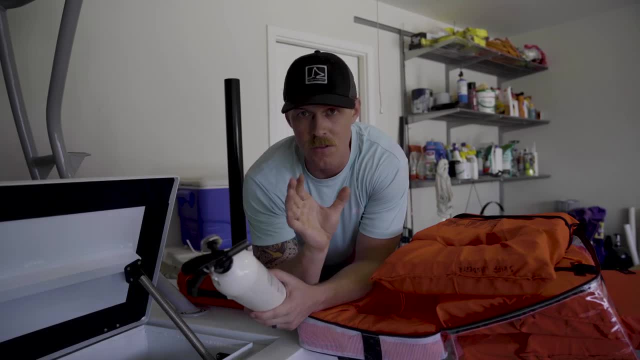 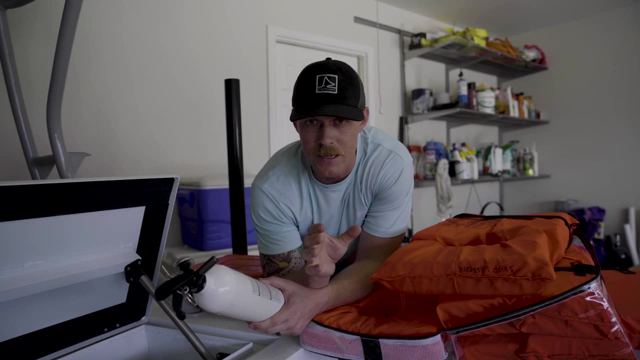 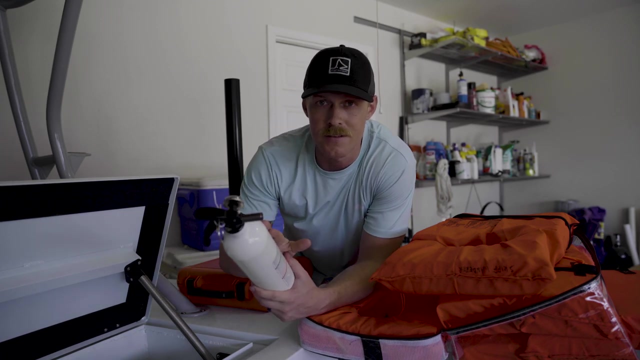 This one is mounted in this rear compartment. You need to look at the state requirements, because they vary depending on the size of your boat, the type of machinery your boat has and whether or not it has fixed firefighting systems on it. Another thing you need to do is, once a year, pull this out, inspect it and make sure it. 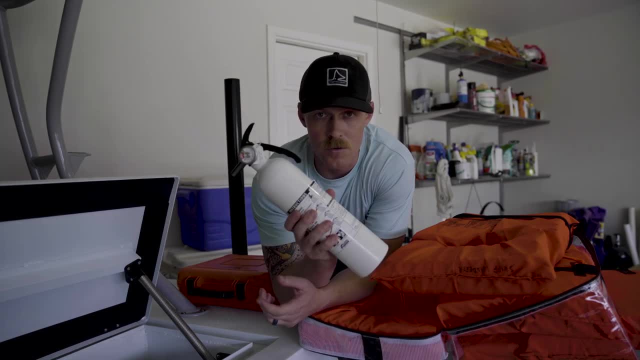 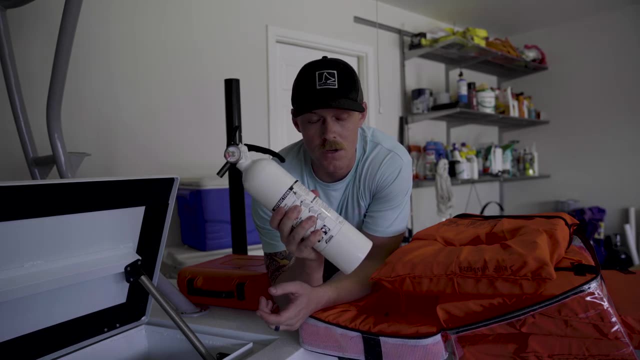 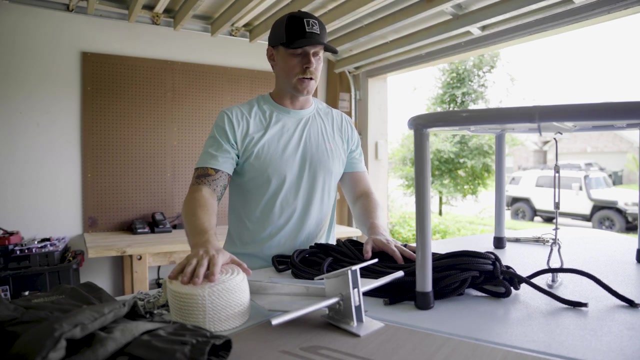 looks like it's in good working condition, The local- Uh, The game wardens can ticket you from not having an extinguisher if this does not look like it works, So keep that in mind, Alright. so the next thing I want to talk to you guys about is dock lines and an anchor. 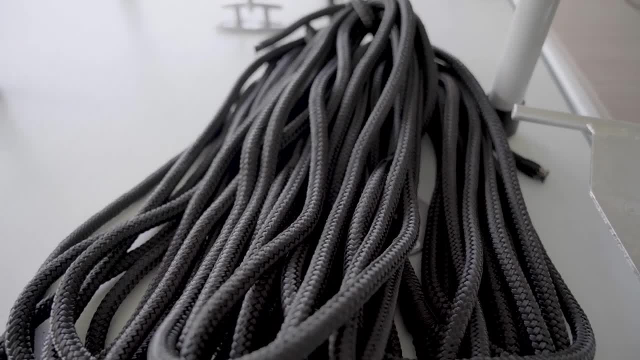 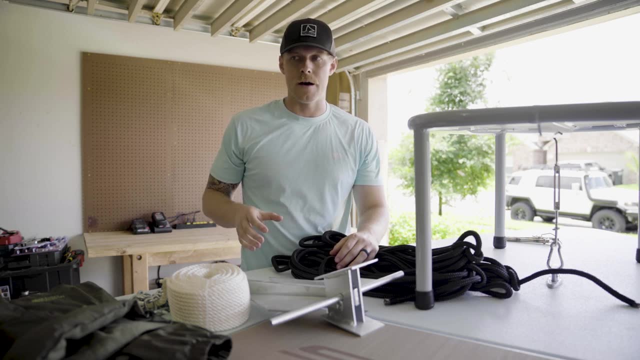 For dock lines, I went with four, three and a quarter inch nylon braided line. Now, when it comes to dock lines, when it comes to how long they should be, the general rule of thumb that I operate by is: you want your dock lines to be longer than your boat. 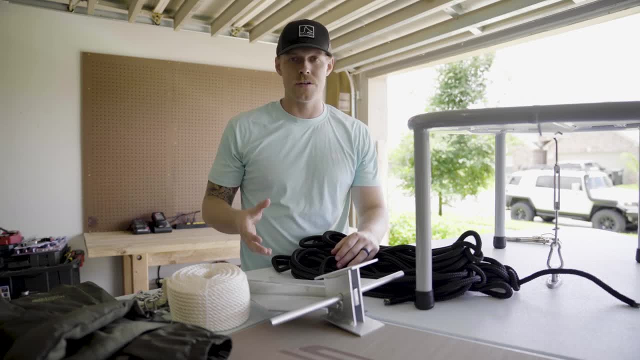 I realize that It probably sounds like overkill, but if you have to dock up and you have a squall coming down on you, you're going to want to be able to double up lines. You're going to want to be able to run long leads so that you can make sure your boat. 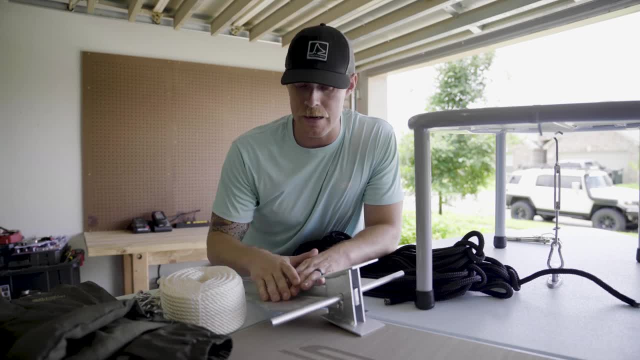 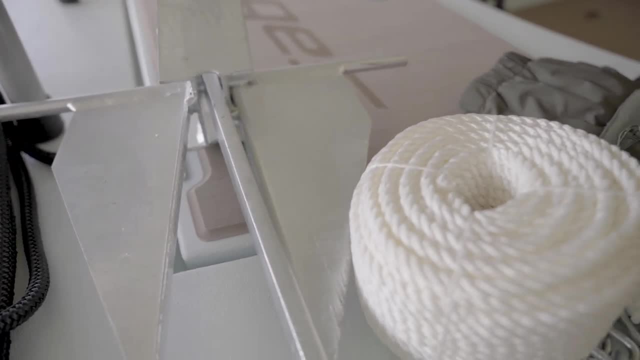 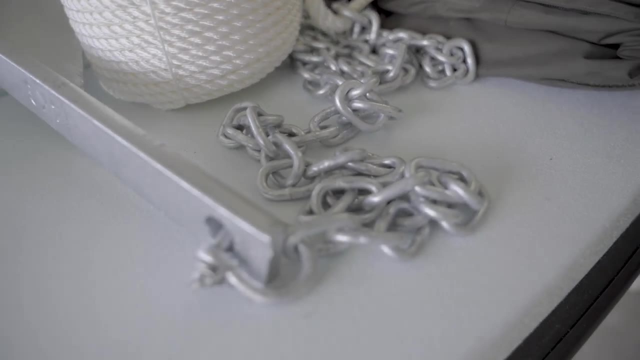 is super secure. Now for an anchor. I went with an eight and a half pound Danforth or fluke style anchor, with six and a half feet of chain and a hundred feet of three strand nylon line. Now, one of the things that I would recommend doing is with your shackles. 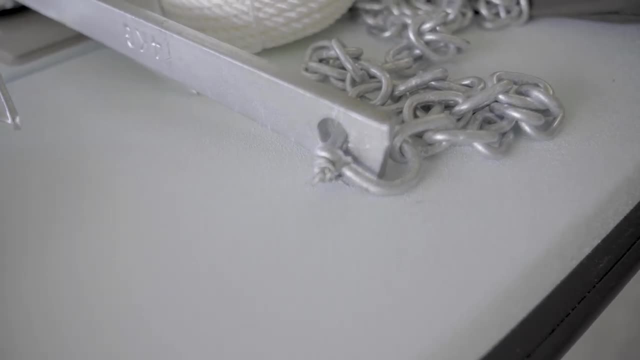 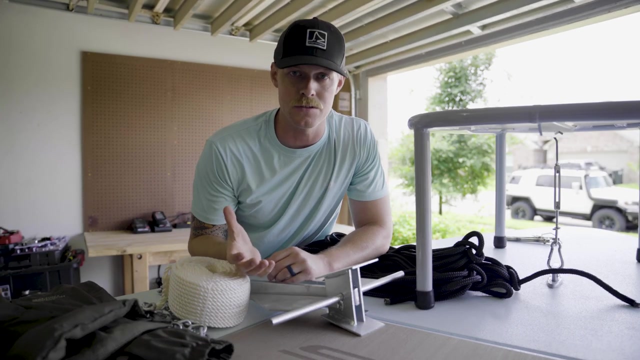 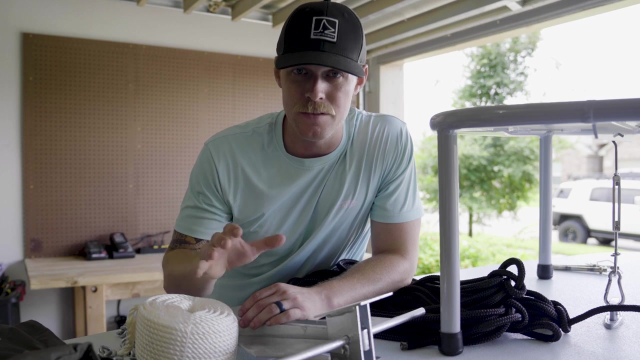 Go ahead, Go ahead and make sure you mouse your shackles, especially if they are screw pin style shackles. The last thing you want to have happen is one of your shackles to come undone. Another thing to think about with your anchor line is it can also be used as a tow rope. 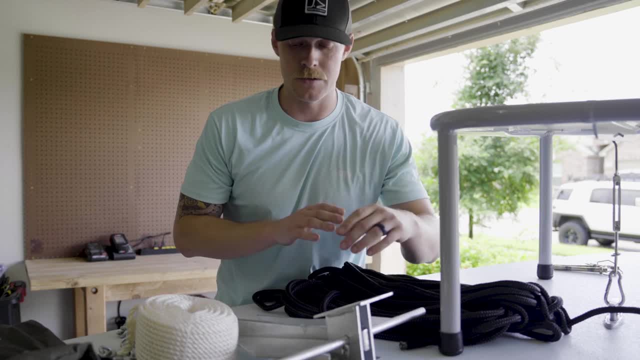 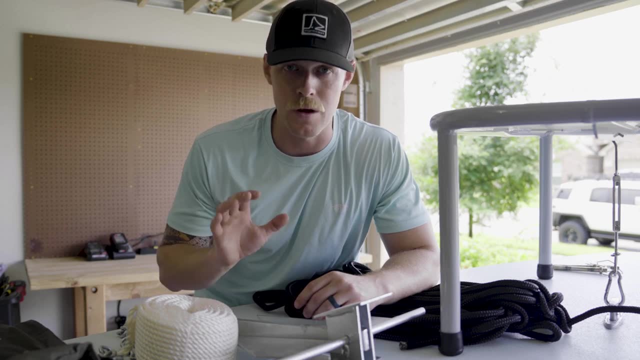 Again, same thing for your dock lines and having longer dock lines. Between these two things, I know I can tie up a towing bridle. if I need this skip to get towed, I don't have to worry about whether or not Someone who's coming to help me has what I need to get towed in. 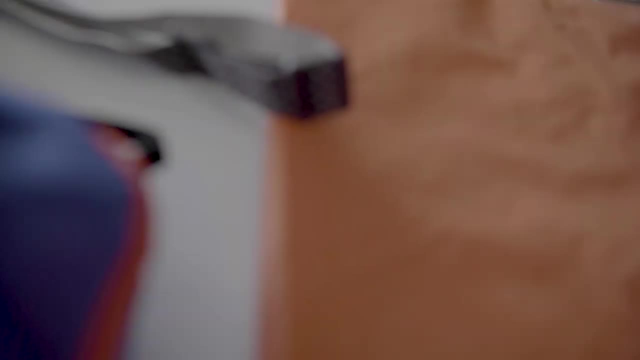 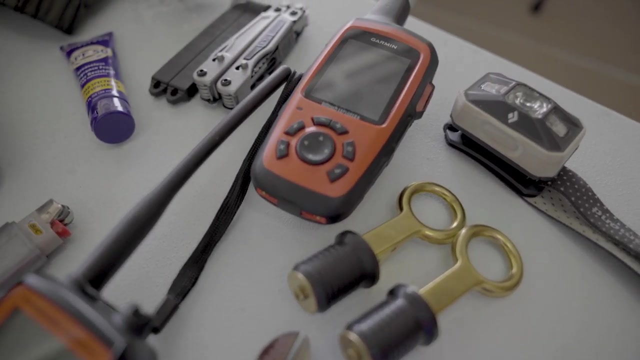 So the last little bit of stuff that we're going to talk about is just spare stuff, extra stuff that I really think that you should have on your boat, Stuff to consider and think about Working in the merchant marine. you're kind of taught to be prepared for any and every. 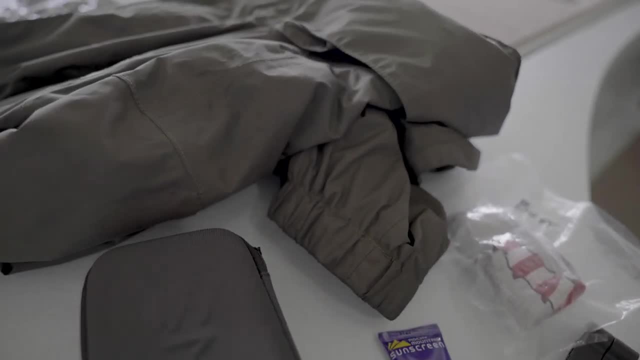 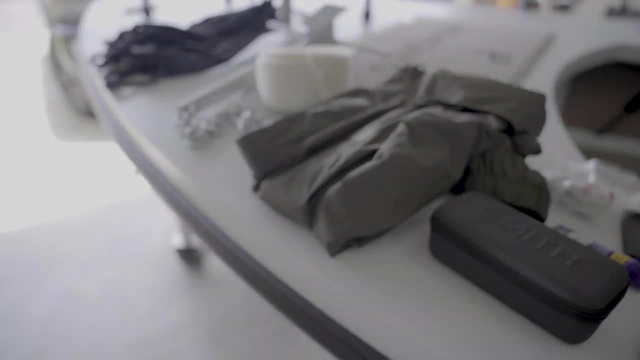 situation and, honestly, out there in the middle of the ocean, there is no help. So I kind of prepare myself whenever I go out on the water- Whether it's on the icebreaker or whether it's on this skip- that I'm going to have everything. 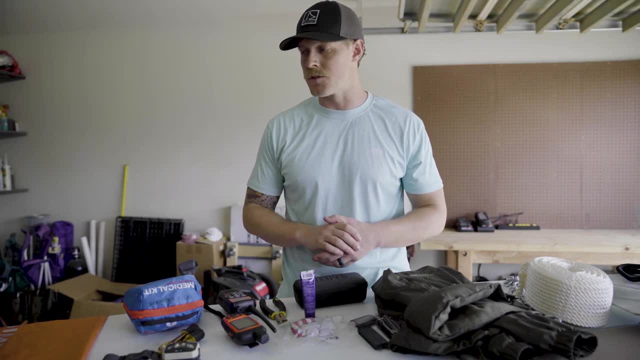 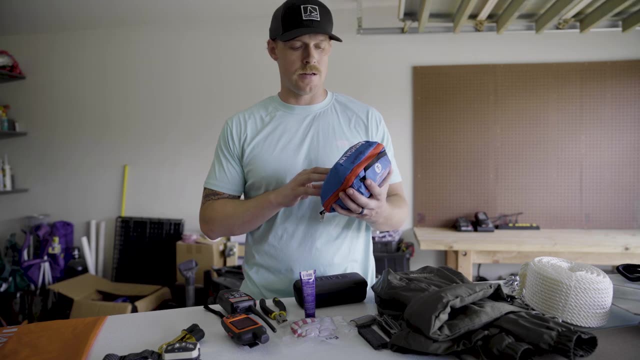 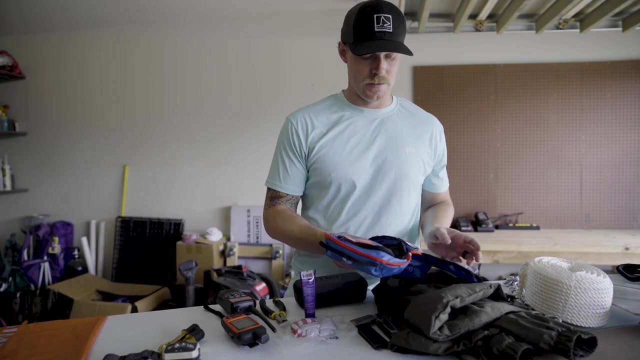 that I need to survive any situation. So, that being said, first things first. first aid kit. Now this is just an adventure. medicals kit mountain series. One of the things that I love about these kits is that they are super organized and 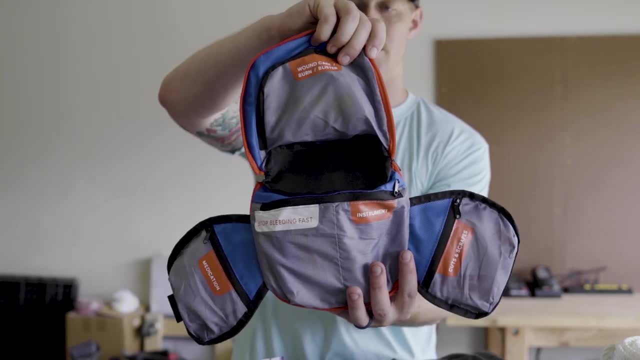 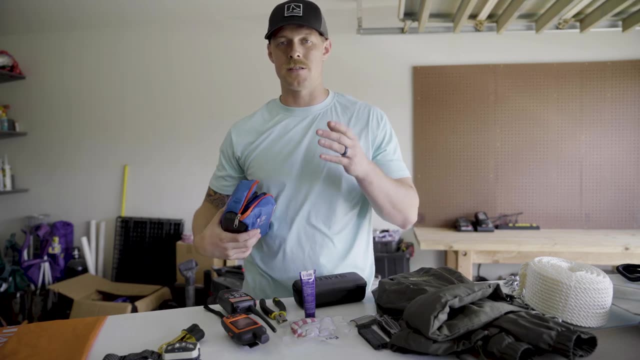 they're super easy to understand what's going on inside the kits. The back of them has a list of everything, The list of everything that's in there. The only thing I'll say with medical kits is: if you're using stuff, make sure that you're. 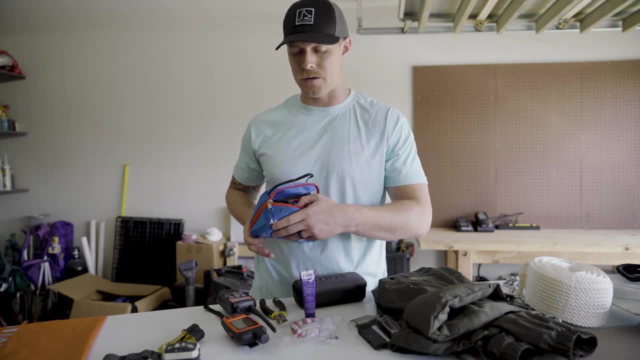 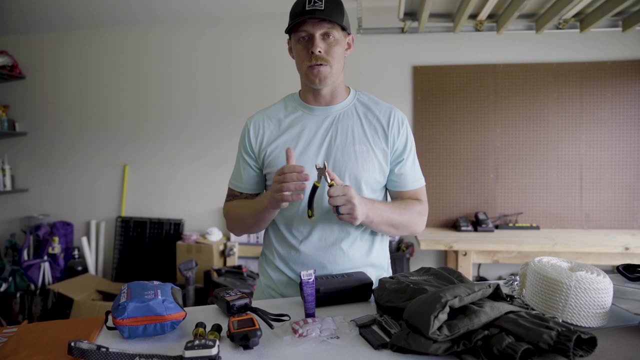 getting back to the dock and you're putting whatever you use back in there, So keep them stocked up. Some other things with first aid and emergency is, if you don't carry cutting dikes with you regularly, it is a good idea to take a pair, vacuum, seal them and keep them with your first. 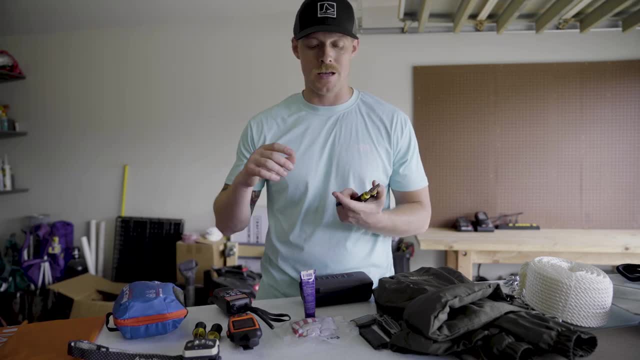 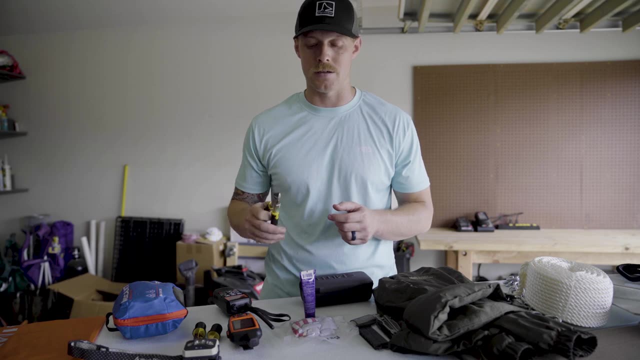 aid kit, The reason being, if someone gets a hook caught in something Inside of them, these things will just cut the tip off and you can get the hook out a lot easier. All right, guys. the next thing that I want to talk to you guys about is communication. 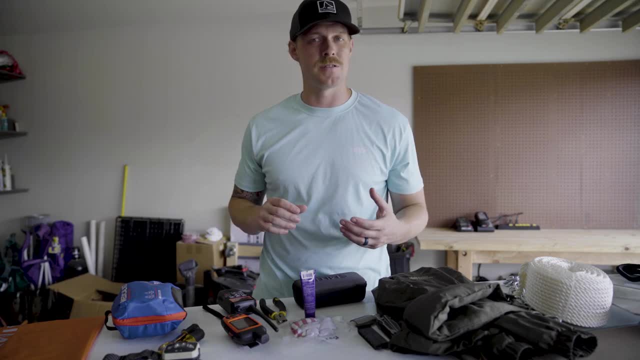 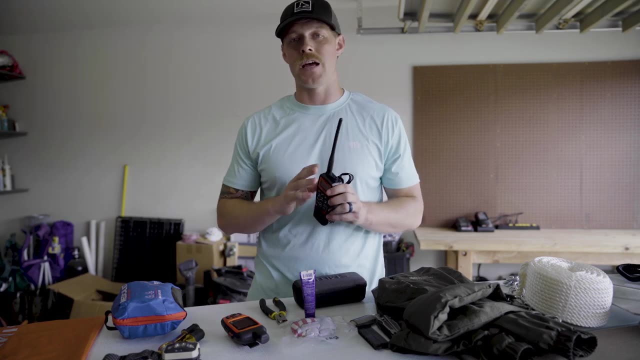 Now when you're out on the water. um most places you should be able to use a cell phone, but it is always a good idea to have a VHF radio. This is a standard. horizon H X two- 10. it is a floating handheld radio. 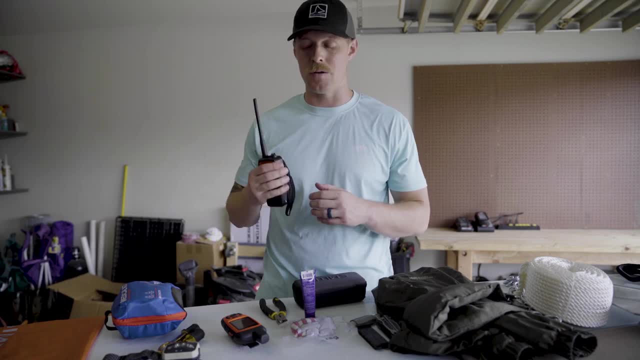 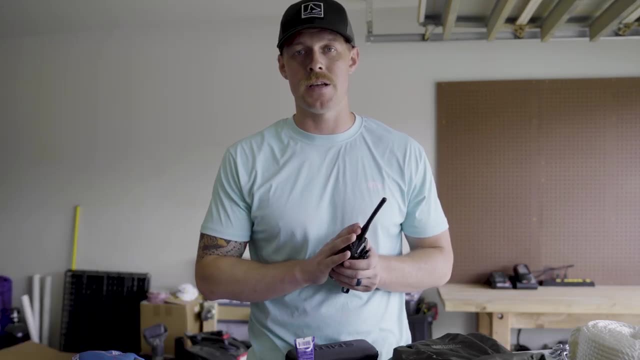 It's got a clip. I can promise you that if I'm on the water by myself, it will be clipped onto my person. That way, if I fall overboard, I can call for help. Another reason you should carry a VHF radio is it is a lot faster means of communication. 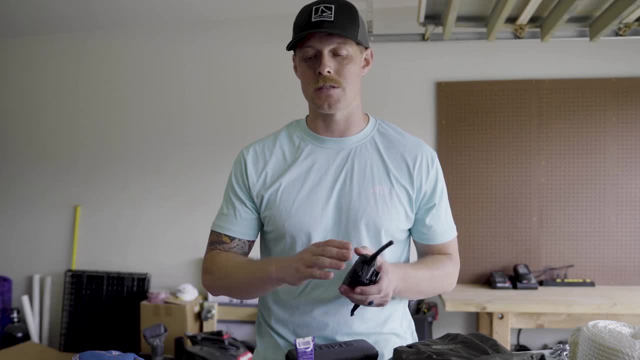 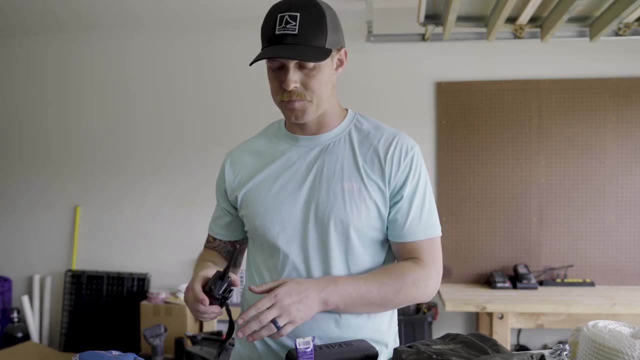 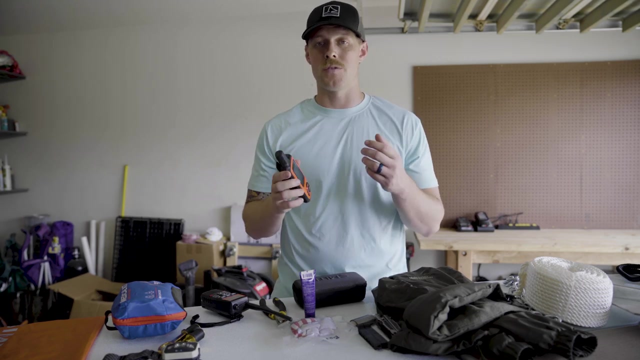 with the United States Coast Guard and with any kind of towing service that will be coming to help you in any situation. Highly highly recommend having one of these with you. The next thing is something like this: This is a Garmin inReach Explorer. Now, I've used this in the mountains. 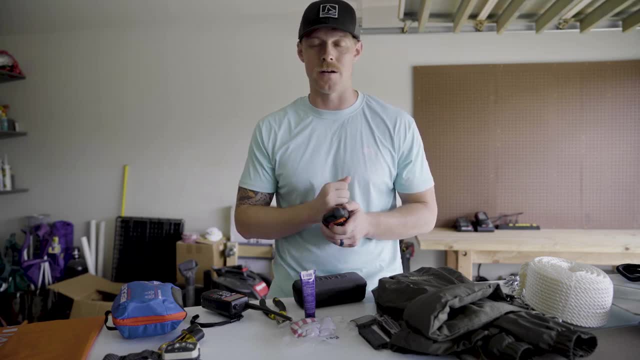 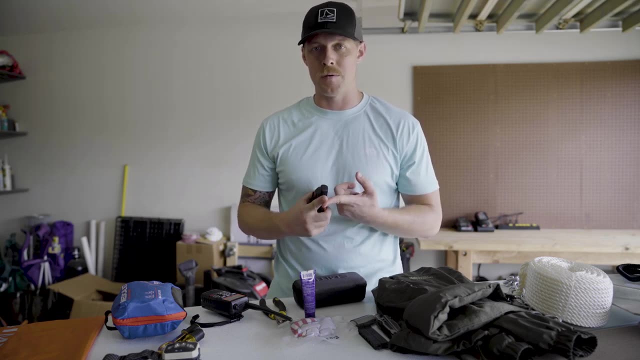 I've got a buddy. He takes this thing to Antarctica and it works down there. The great thing about these is they can send your position at whatever time interval that you choose. Um, if you're in an emergency, you can just hit this SOS button and it will notify the. 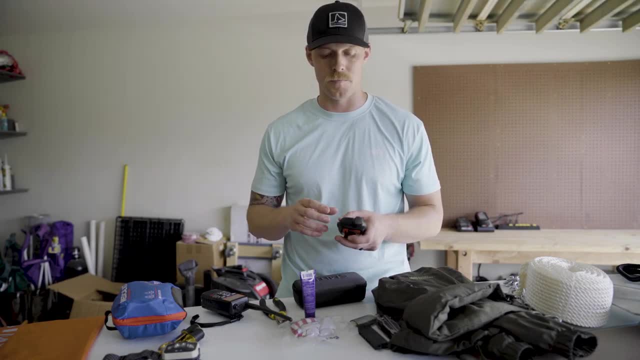 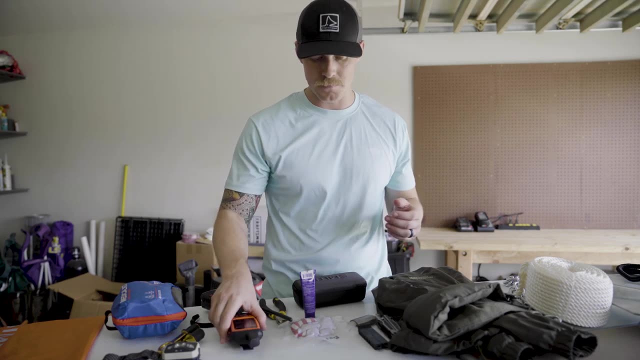 local authorities that you're in trouble and it'll start getting rescued to you. Um, also, it's a GPS, so you can use it to keep track of where you're at. All right, The next kind of things. This is my kit that I like to keep on the boat. 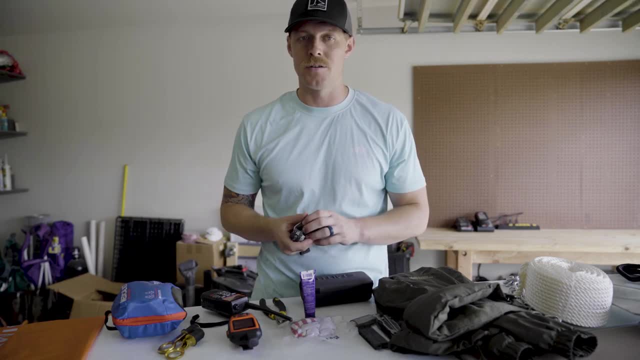 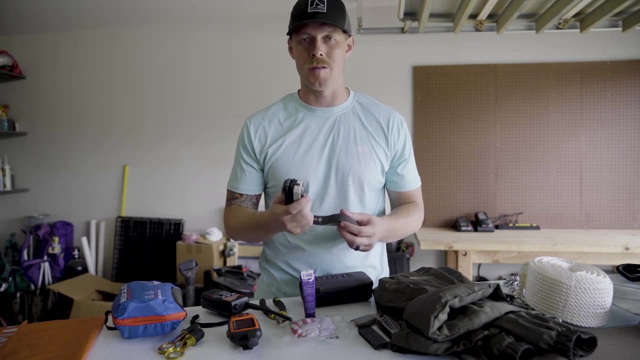 Um, headlamp Flashlights are great. Your phone has a light, that's great, but more times than not you're going to need both hands, So having some form of a headlamp on the boat is going to be really good for that. 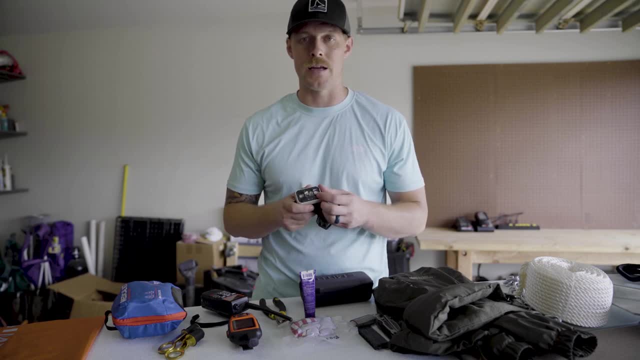 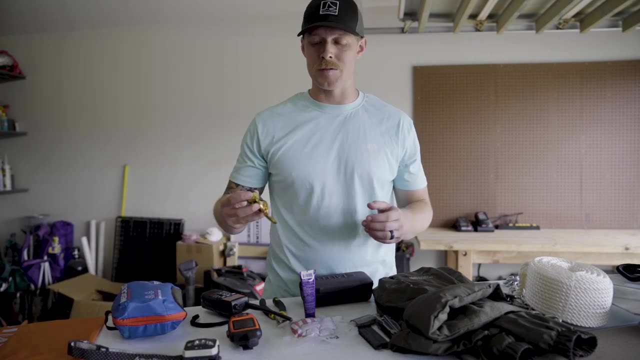 Uh, another thing to keep in mind is, if you're going to have any kind of light that uses batteries, to make sure you carry spare batteries on board. Um, speaking of spares, spare boat plugs. Now, This requires two boat plugs. 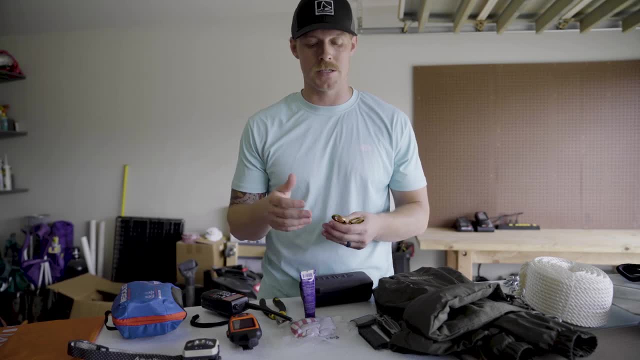 Um, I'm going to keep two spares on the boat as well in my ditch kit, And the reason for that being is: two is one, one is none. So a good idea to make sure you have a spare boat plug, because without a boat plug, your 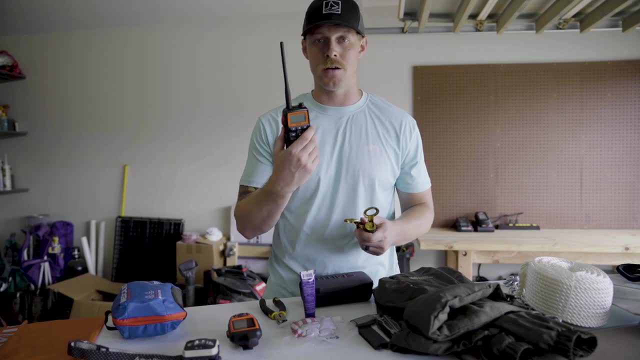 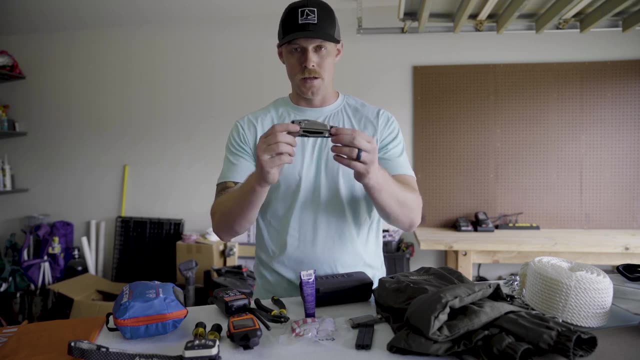 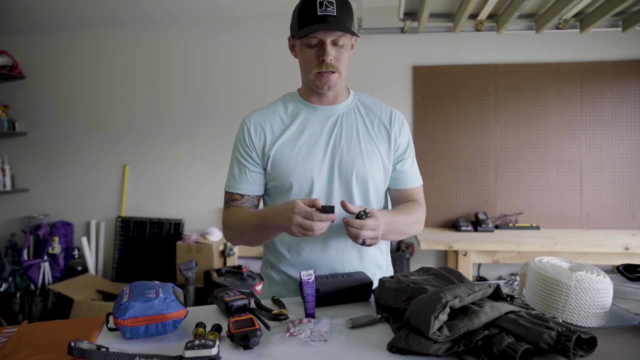 boat sinks, and then you have to use your radio to call the Coast Guard. Also, along the lines of um tools and equipment, Some form of multi-tool is a good idea. Um, I really like this SOG one because it can take bits inside of it. um which will. 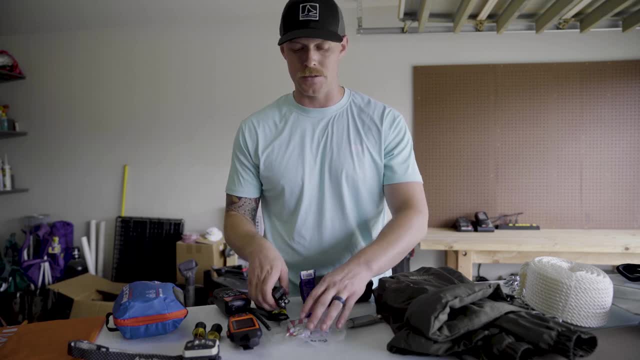 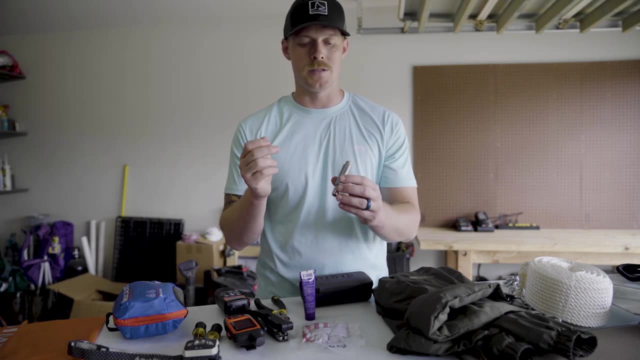 allow me to work on any kind of mechanical issues if I need to. I also like to keep a lighter with me, and I tend to wrap my lighters in duct tape, which this will give me a good 30 feet of duct tape if I need it. 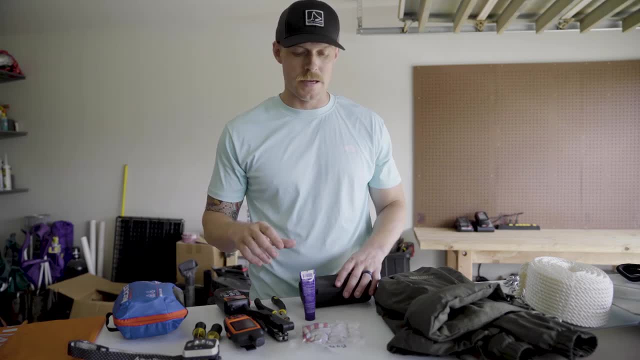 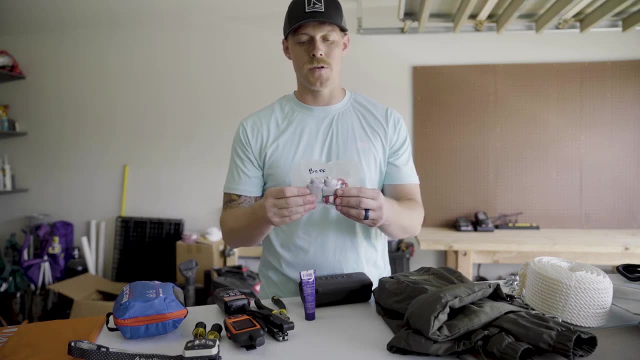 And we all know that duct tape fixes everything. Lastly, Some things that can make or break a day on the boat. Okay, If you're out on the water, uh, spare buff, this will keep the sun off of you If you forget one. now you've got one on the boat, you don't have to go back home and it'll. 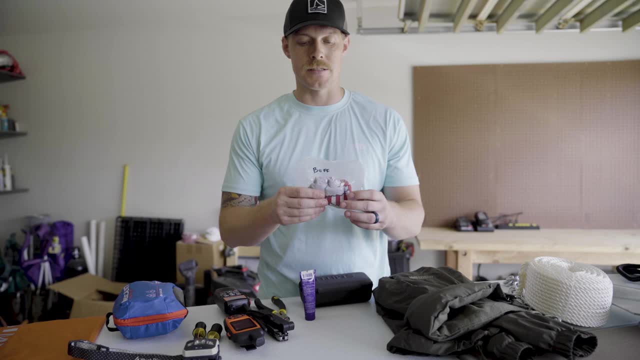 make your day a lot more enjoyable. Um, I would like to take it and vacuum seal it. This makes sure this will help keep it dry and I can just leave it in my bag and I don't have to worry about having a wet buff. 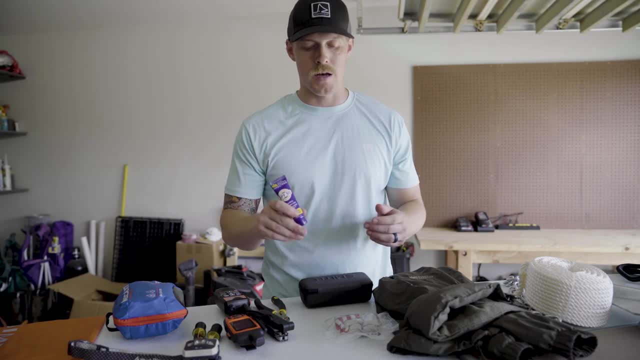 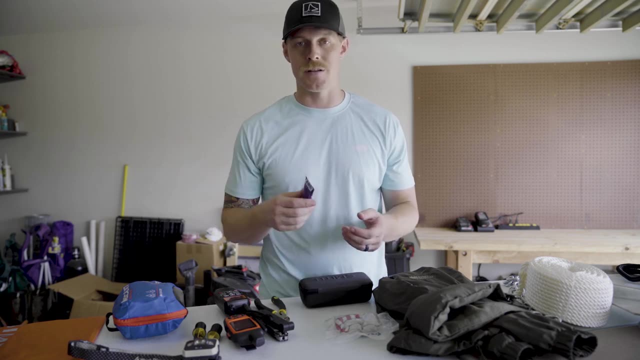 Spare sunscreen. I like to keep a small tube of sunscreen uh with all my spare equipment, just in case I decided to forget it. My sunscreen in the truck, which, to be honest, I do a lot of. uh. spare sunglasses. 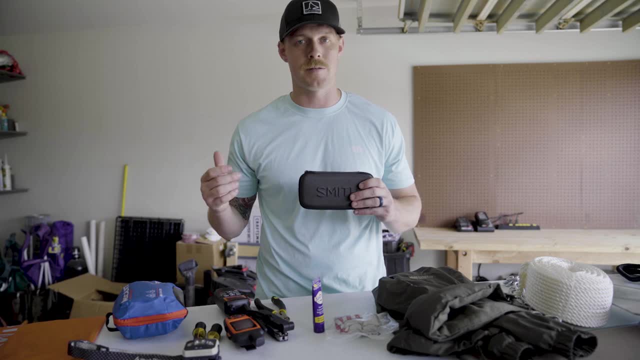 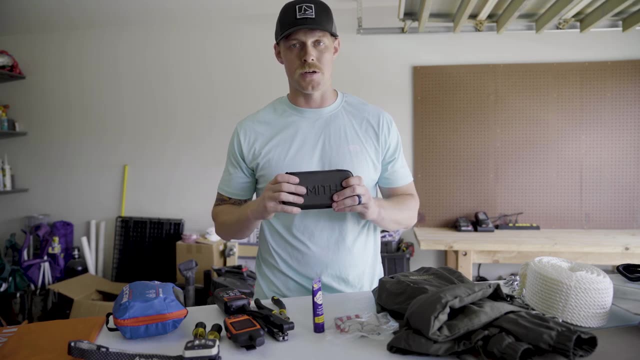 I like to keep a spare set of sunglasses on the boat in case somebody loses them, in case somebody forgets them. especially fishing, You're going to need them, So make sure to have a spare set on board. Rain gear- Summertime. 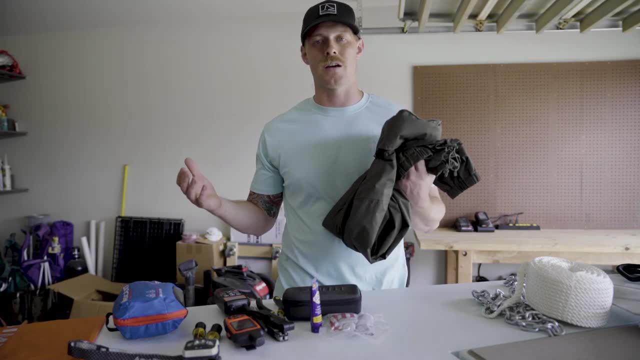 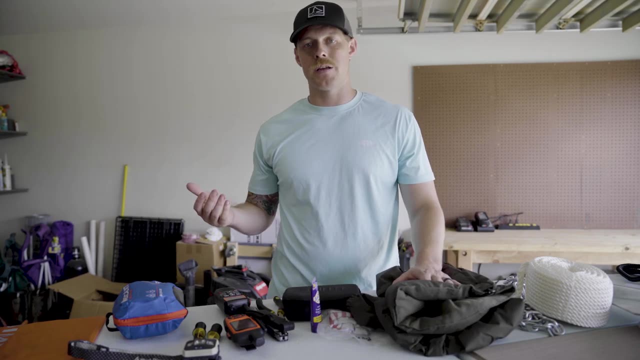 I'll just throw an extra rain jacket on the boat. Even if it's not calling for rain Wintertime, I'll throw rain pants on the boat And, honestly, having rain gear can make or break a day, and it can really keep you from. 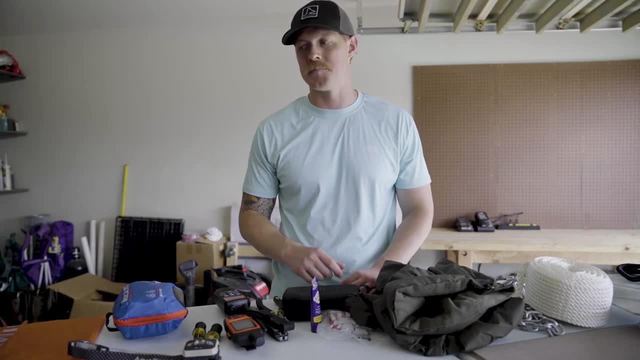 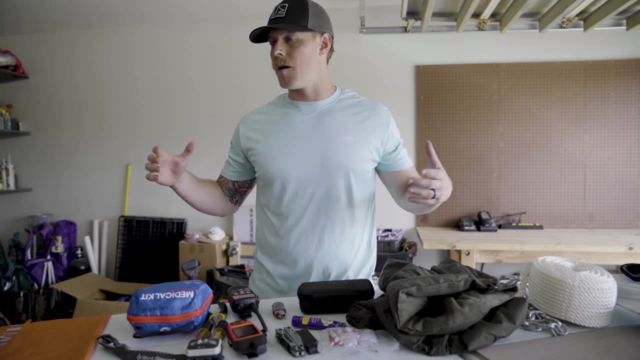 having a miserable, miserable, cold boat ride home Now. the very last thing that we need is something to put all this in. Um, obviously, it's not all going to fit in the same thing, but I recommend some form of a dry bag. 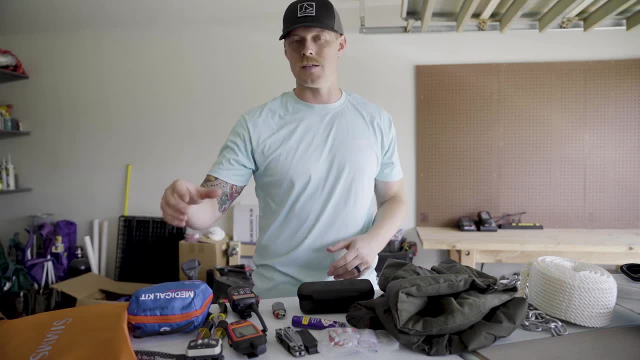 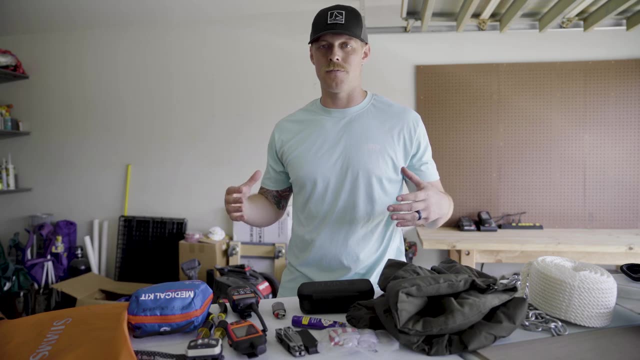 Um, hard cases work too. The reason I like dry bag is you can contain air And I'm rolling them up, clip them and then they float, which, if your boat goes down. you want as much stuff floating around you as possible to become a bigger target for. 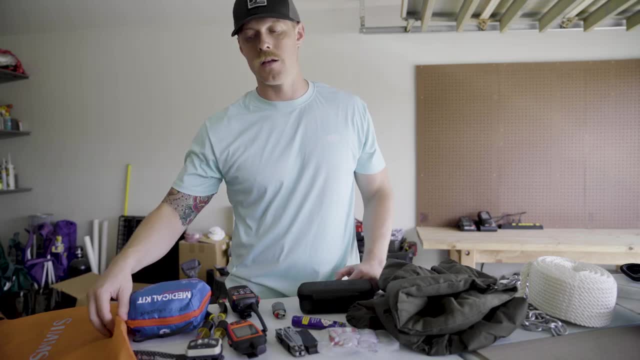 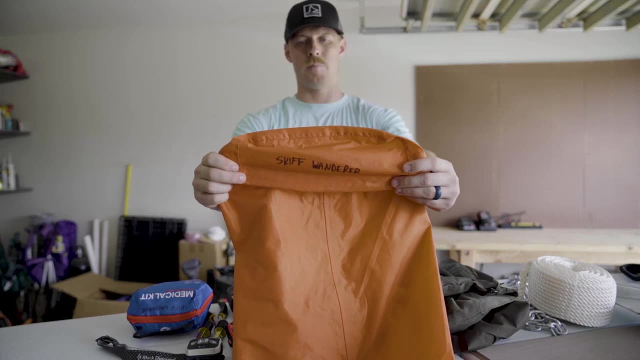 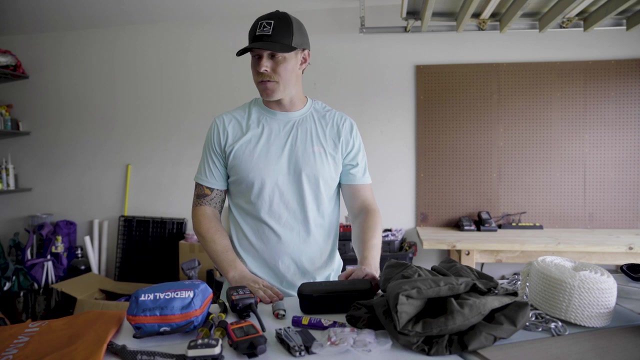 your rescuers to see. So that's why I went with a orange dry bag and again went ahead and put my name on it. Now it looks like that's all the stuff I've got, So I guess, uh, Time to load the boat up.